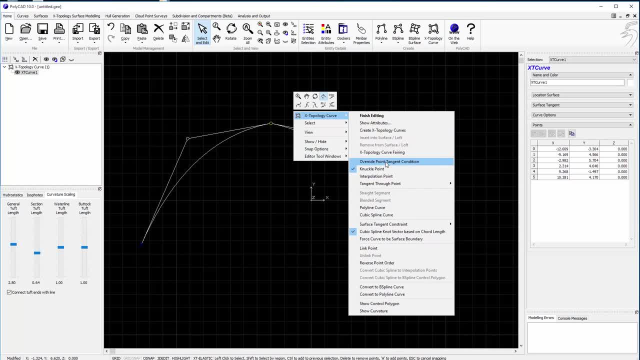 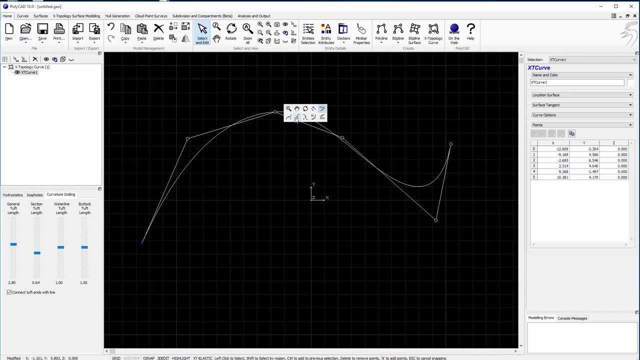 and these are also reflected in the options down here. So we can add a knuckle point, we can make that an intersection point, we can give it a Y tangent, So there's lots of different sets of curve level tangencies. We can also insert a straight segment. 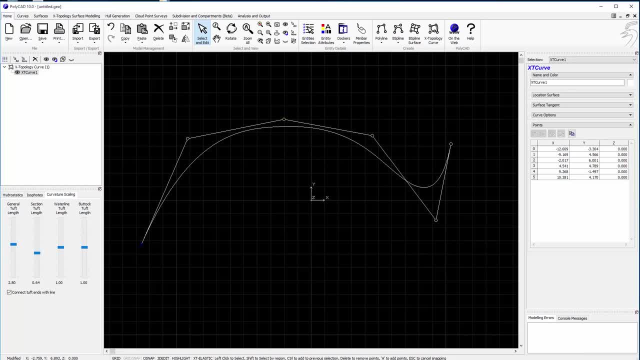 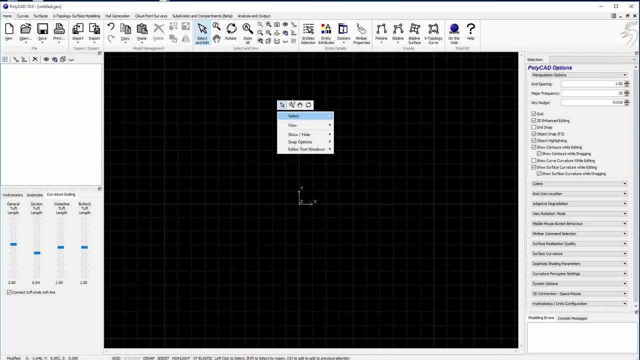 We can also import or specify blend, So it's as simple as just designing your curve, and that's ultimately where the whole idea of design intent comes from. So therefore, making something like a midship section for a ship is pretty straight forward. So if we just 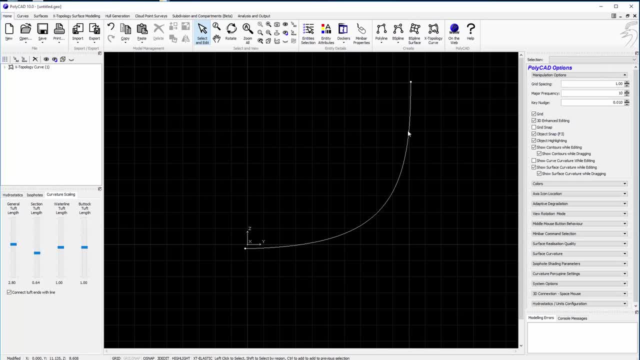 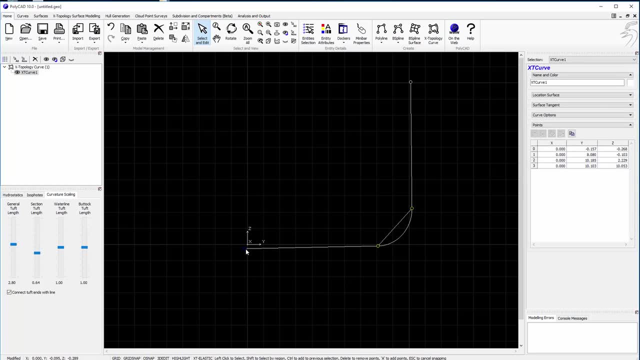 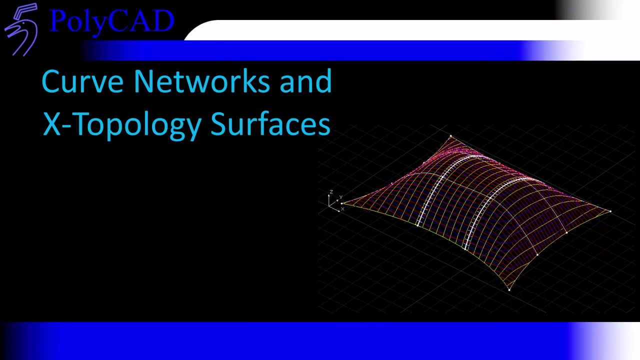 draw points. All we have to do is put in a blend and we had a midship section. If we use the grid now we have a tidy midship section. Now we'll go on to use the curves to make a curve network and to use that network to define the next. 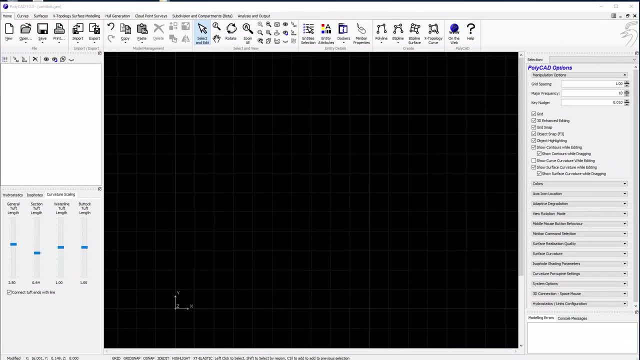 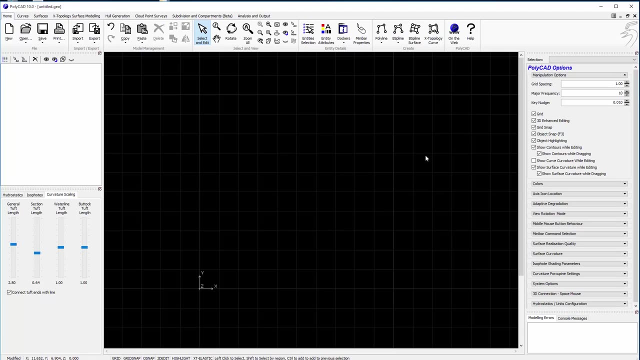 topology surface. So one of the important characteristics of X topology curves is the ability to build a curve network, and for this we kind of combine the snapping facilities of PolyCAD with the dynamic kind of attachment capabilities of the X topology curve. So we'll start out by drawing a simple square of curves and if 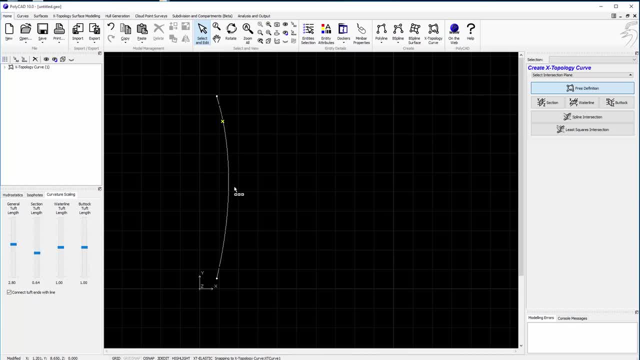 I now continue to draw curves. obviously, we get the snapping feature that we get with all curves, but the difference here is that we get the set of links shown that indicate that the curve will be connected together. So we can create a curve like that and like that. Now, if we 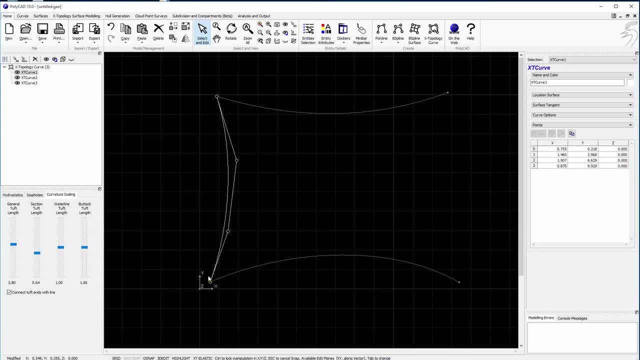 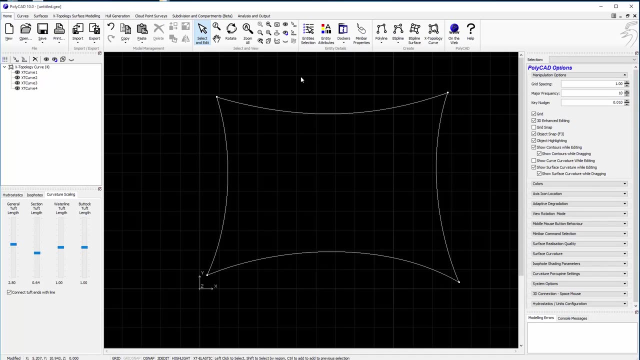 go back and edit the initial curve. because they're linked together, you get the dynamic capabilities all coming into play. It's a nice way of- again like with the attributes- setting up some design intent, creating a master curve, and all the child curves connect together. So now I have a 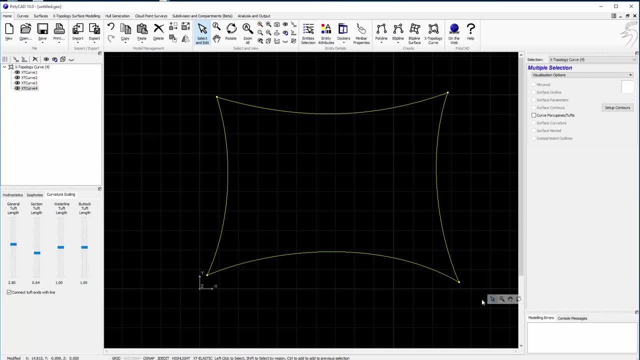 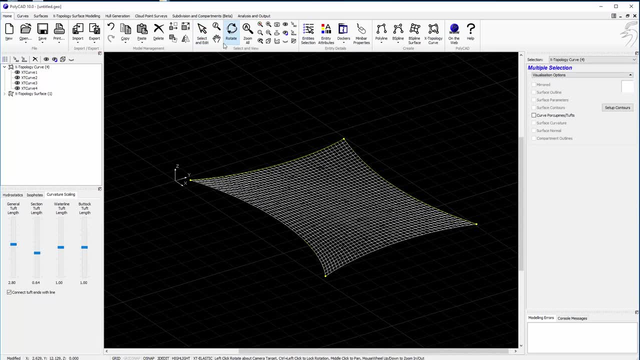 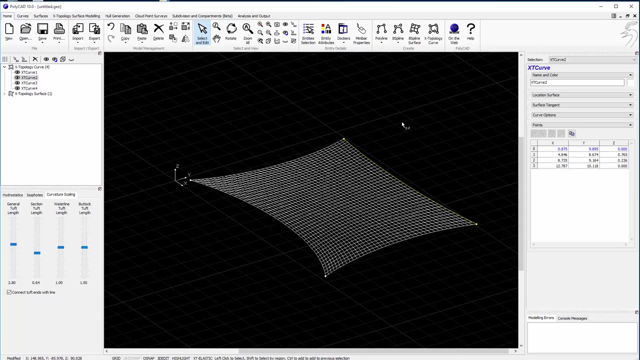 rectangle. now I can go on to make the next topology surface, So selecting all the curves. I can bring in a surface that way, Because everything is dynamically linked: as I move the points around, everything will update. Now that's fine, I can go on to build a more complicated surface. Let's add some. 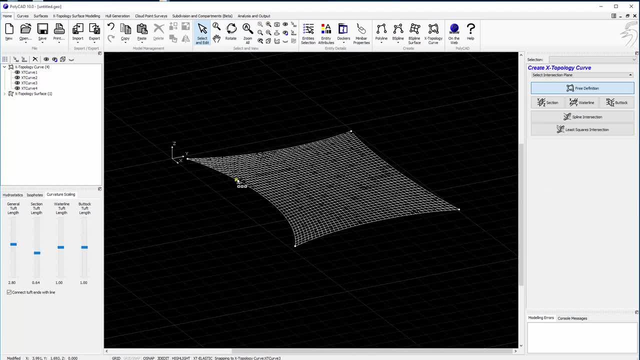 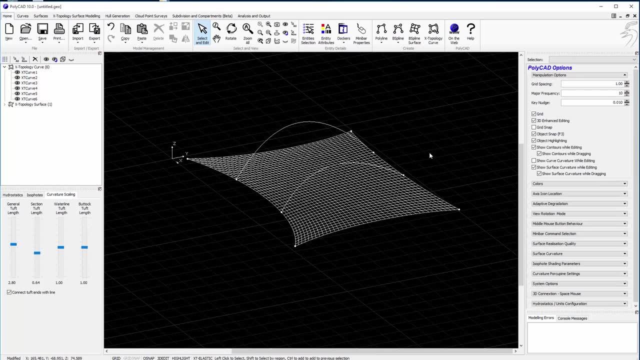 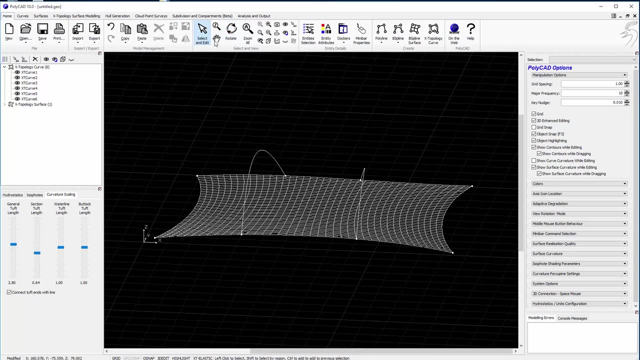 sort of sectioning effects in. So let's add a couple of curves across the shape. At this stage they don't get inserted into the shape itself. Let's do a little bit more. so let's make these plainer curves. If I set them to be plain in the 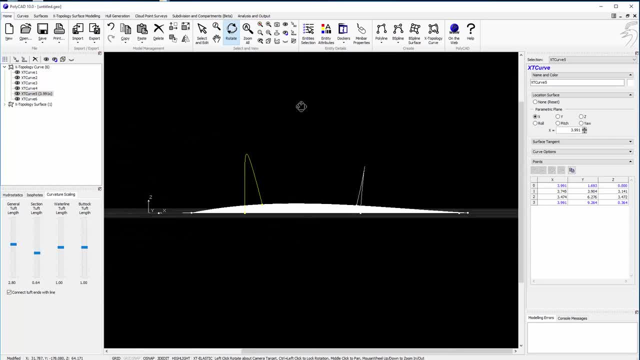 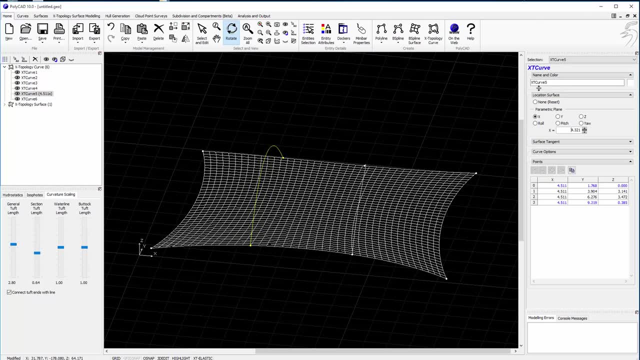 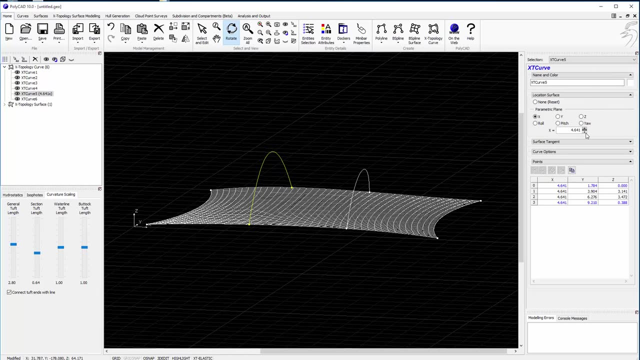 X, then their position is now different. find in the X location, or at least it should be. It's taking us a little time to update, but now with an X plane it's got the option to be all driven as one shape. We'll do exactly the same with the other curve. So now to insert those. 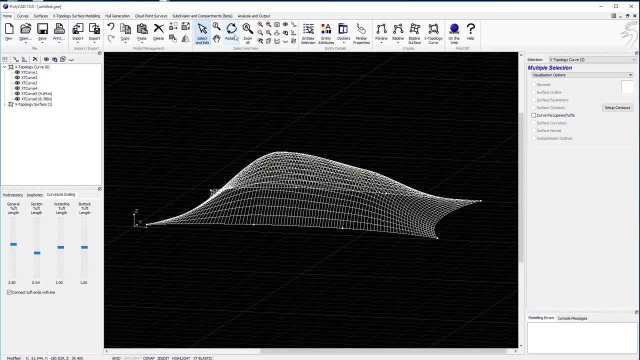 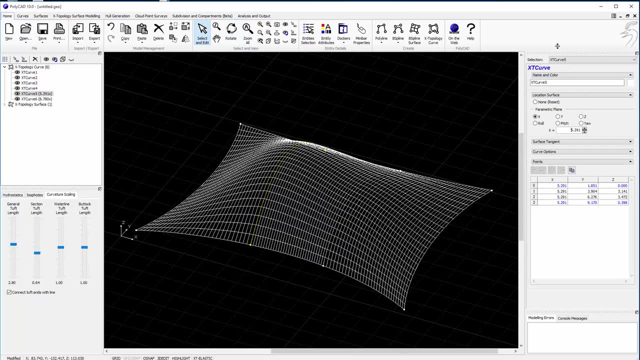 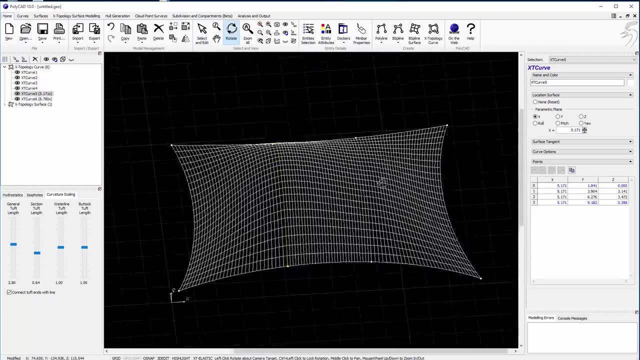 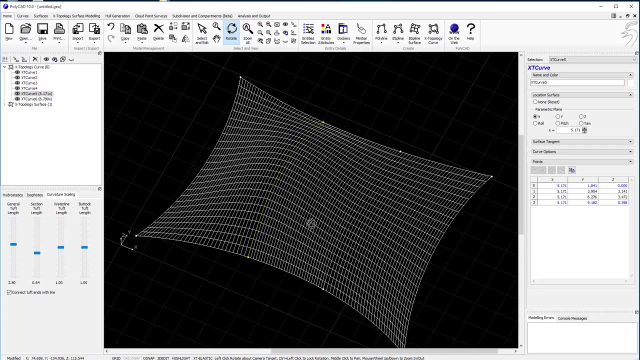 into the surface. we'll just do an insert. You can now see the surface now gets the shape of those curves and again, if we move them to the surface, updates. Challenges with this kind of approach is that everything, all the curve tangencies, are being interpolated along the length of these, so we don't always get. 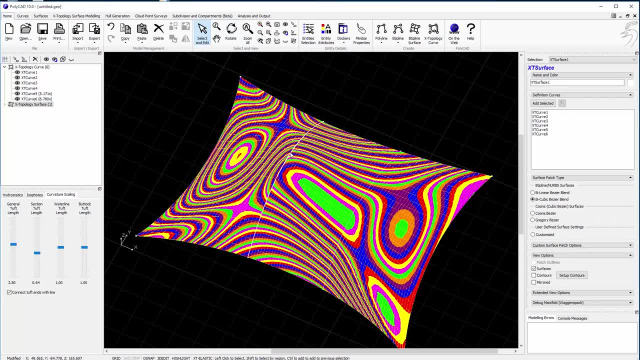 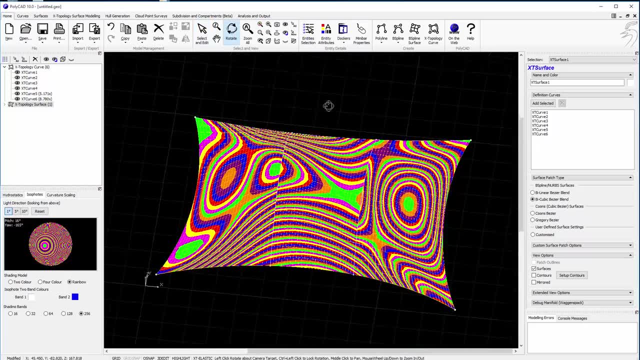 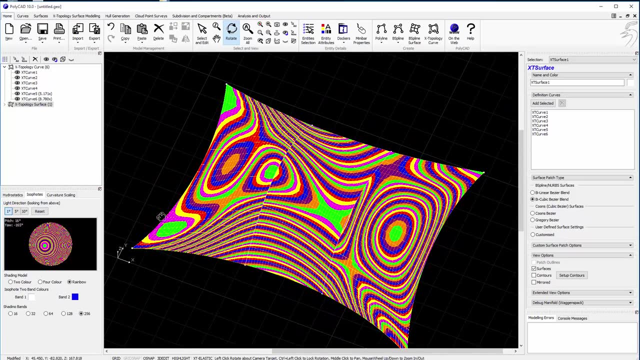 completely perfect curvature. You can see here we've got, if we look at the isofocs, quite a breaking curvature, and this is just down to the fact that the surfaces themselves don't have enough mathematical information in them to achieve that continuity We can prove. 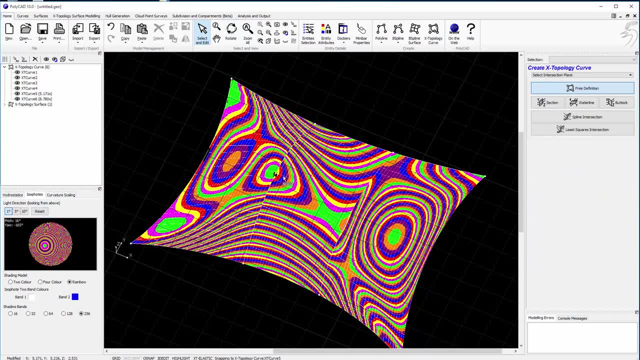 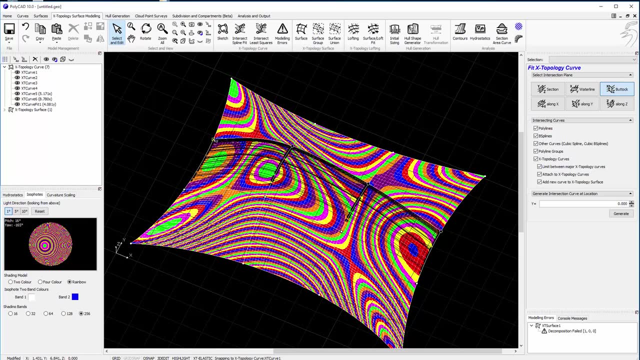 that by adding an X topology curve in the other direction. Now here I could just draw it across the surface. but if I use the spline option and we'll take a buttock line, then I it can be drawn across the surface in one go and you see. 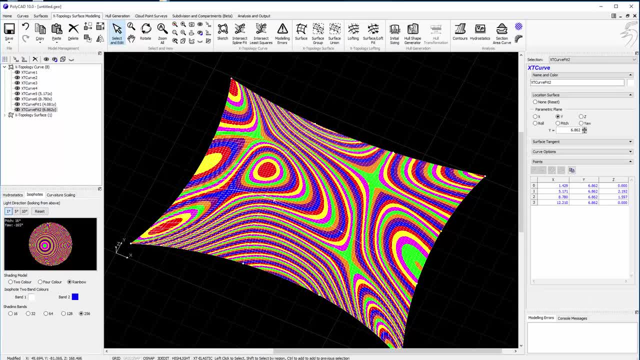 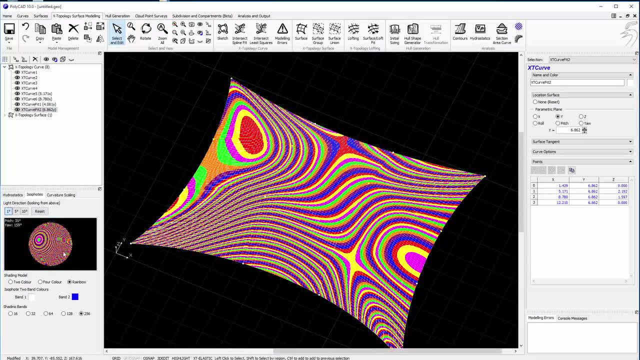 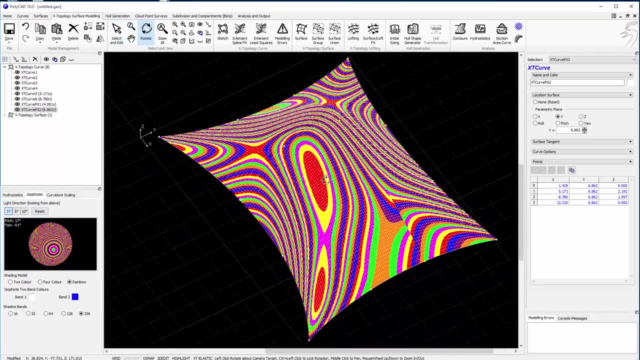 As I do that. I've drawn two curves there. The continuity improves as it's drawn across the surface. You can still see we have some lower area there. We've got some break in the surface. That's just down to the way that the mathematics work. 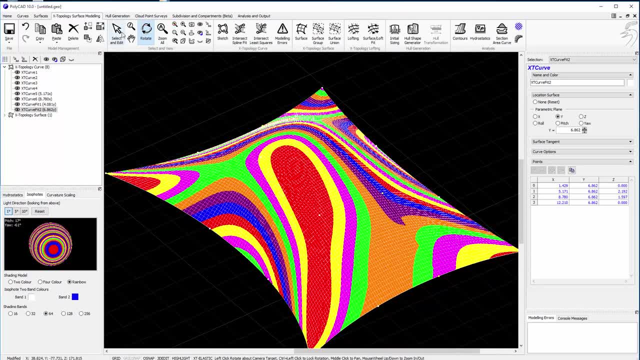 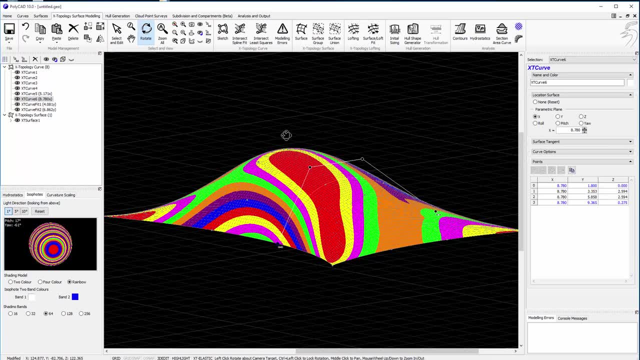 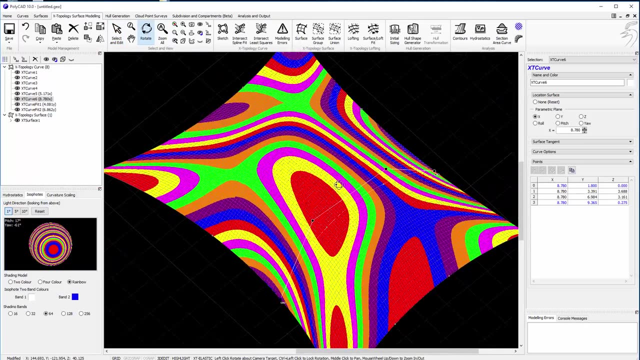 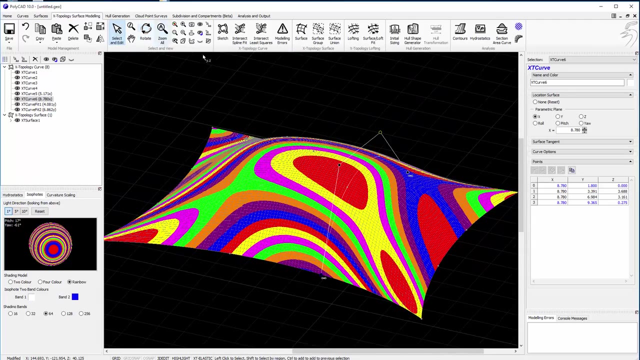 Now that we have a smooth surface, you can edit the curves. Sometimes you might want to take snapping off If we're not wanting to snap, but we just want to edit. there we have a surface like so If we wanted to change the role of that curve, we could make it into a knuckle line. 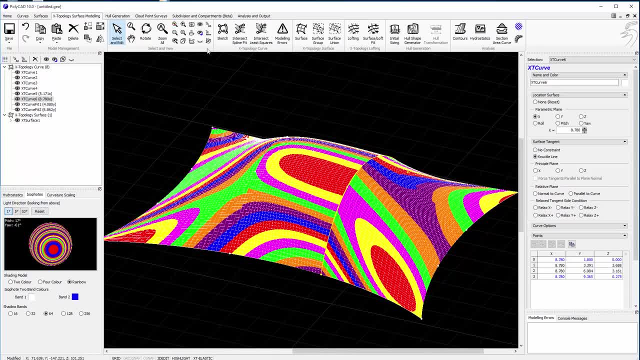 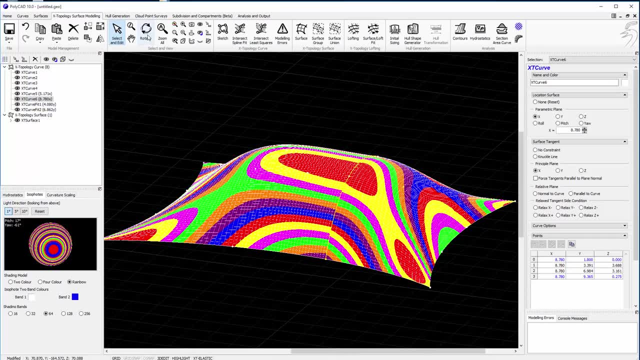 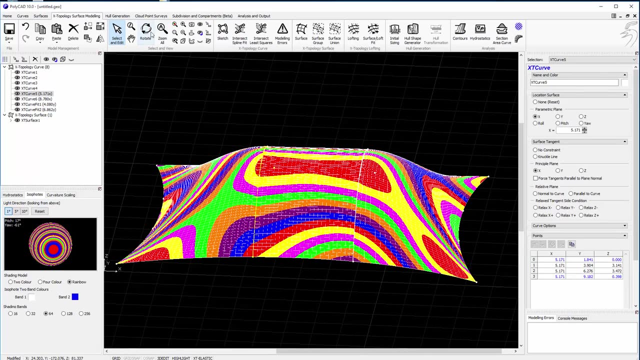 This is where some of the surface tangency options come along. Make it into a knuckle line. We have a direct corner. We could turn it into a X. Now it's enforcing an X tangency in that direction. similarly for the other curve. 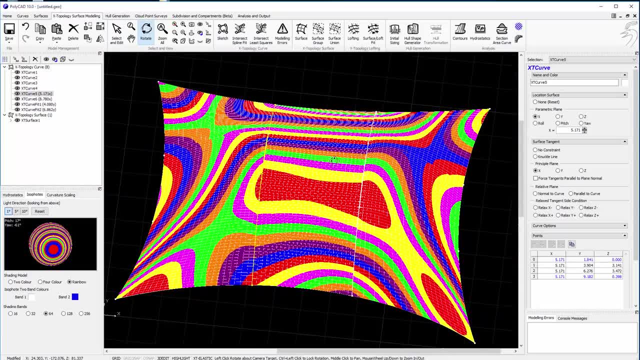 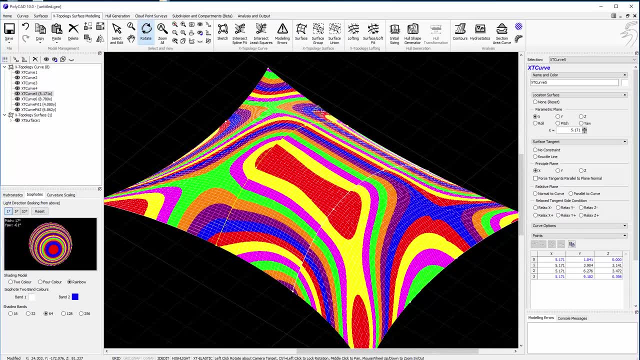 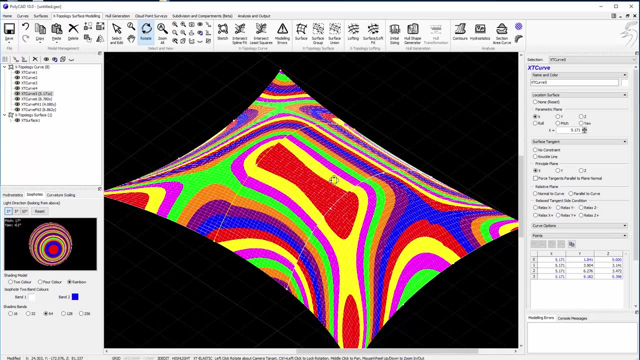 We start to get a linear effect along there Because it's enforcing tangency, then there's going to be a break in that shape. With this we can start to define the limits and shapes, specifically by giving characteristic information, by adding constraints to our surface as we go through. 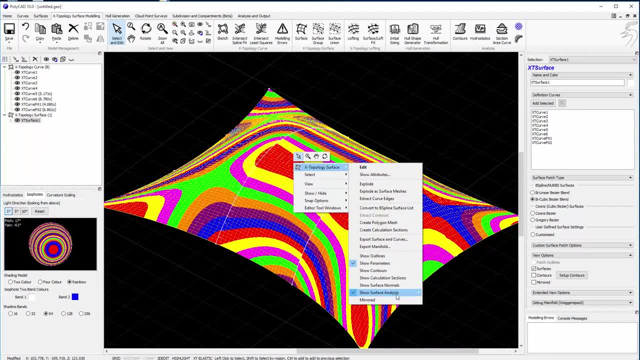 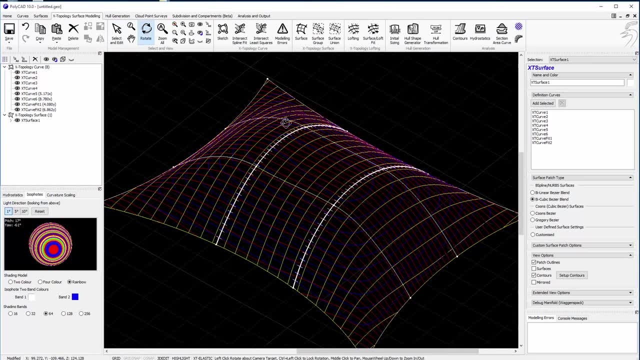 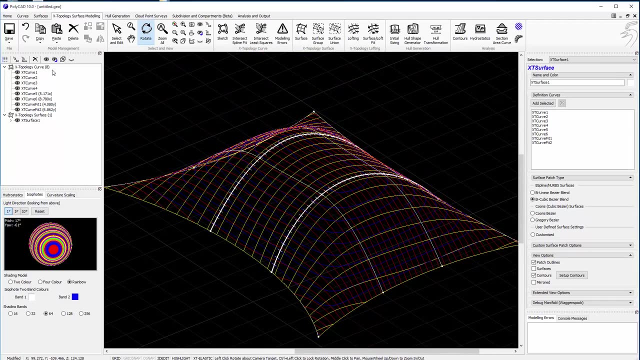 Thank you. Of course, considering that we're designing a hull, it's very easy then to set up contours. We can see standard shapes or standard output that we're expecting. If I was to, for example, again draw a midship section, I'll draw the section earlier I'd. 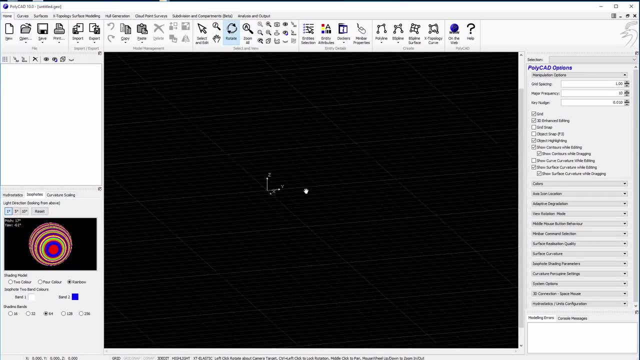 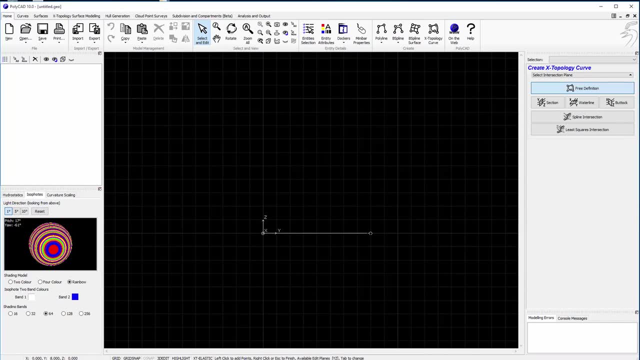 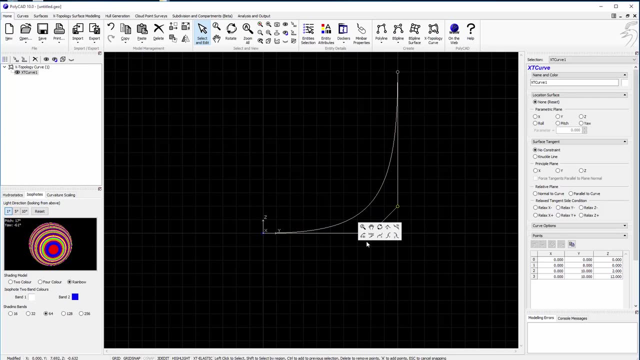 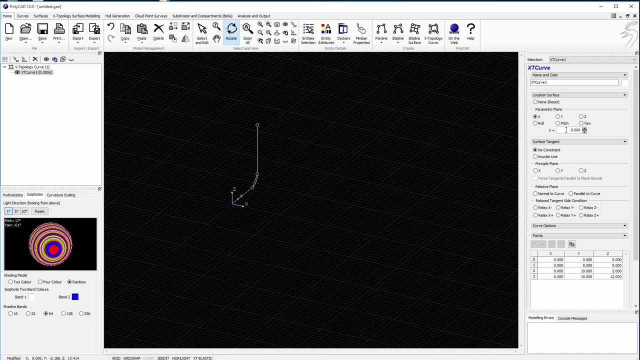 probably use the following approach. We could start out, say, by looking in a section view. Okay, Let's start with our grid on Drawing a curve. We'll now edit that to add in the build radius. Of course, this curve is located at the origin, so if I add in, make it a planar definition. 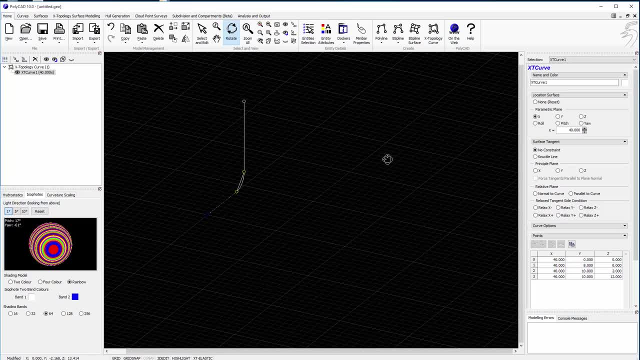 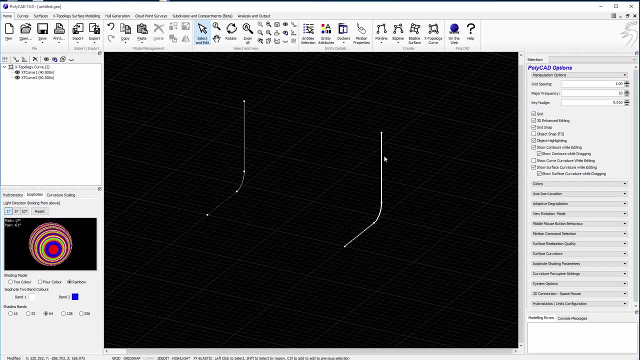 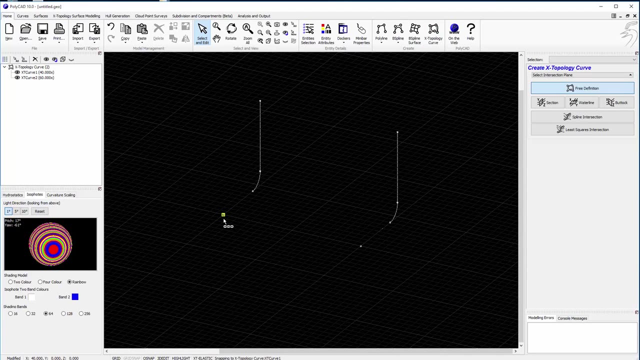 move that to 40 meters and obviously we're going to create an extrusion here. so why not take a copy? Okay, There we go, There we go, There we go. Now I have two curves Now, adding on our constraints again and our snapping. we'll just connect these up.